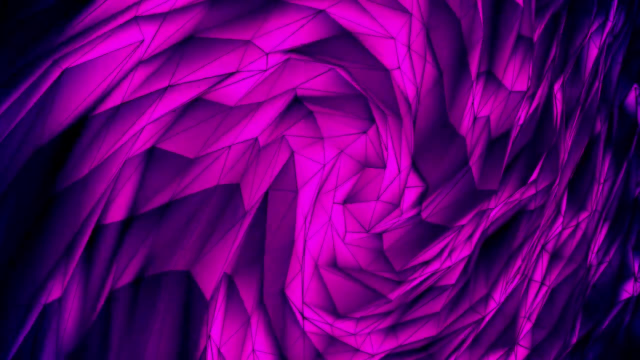 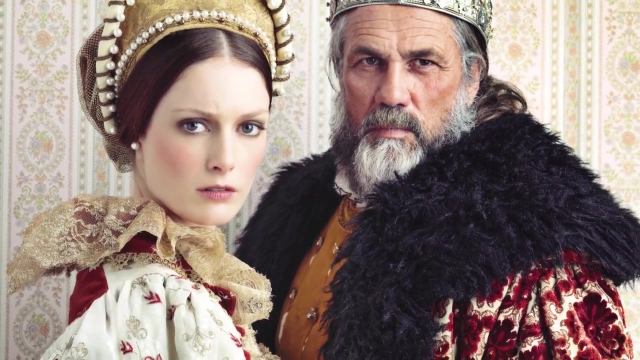 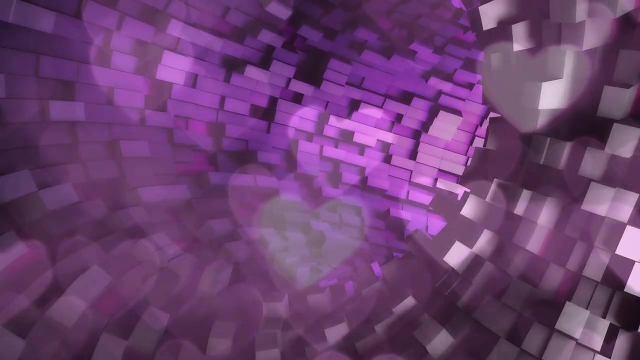 Purple is also associated with royalty because it was one of the first colors used by kings and queens in Europe during the Middle Ages, when they had no access to other colors like red or blue-green, the latter being associated with good fortune. Purple is associated with wealth, luxury and opulence. 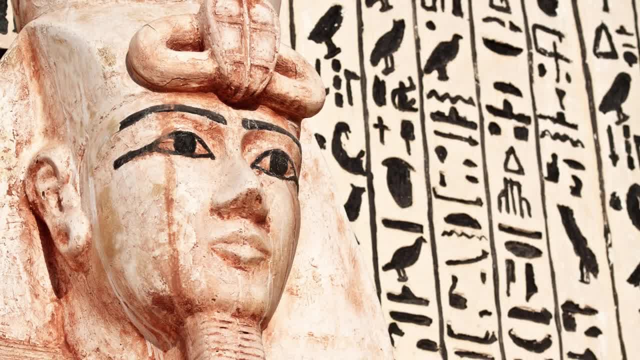 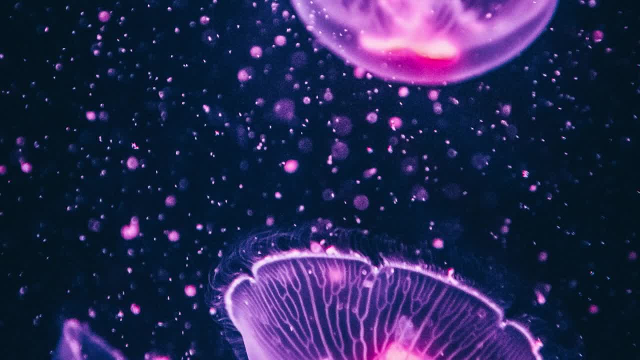 The color purple has been a symbol of royalty for centuries. In fact, it was the color purple that was used to symbolize wealth, luxury and opulence. The color purple has been a symbol of royalty for centuries. It was the color worn by kings and queens in ancient Egypt, Greece and Rome. 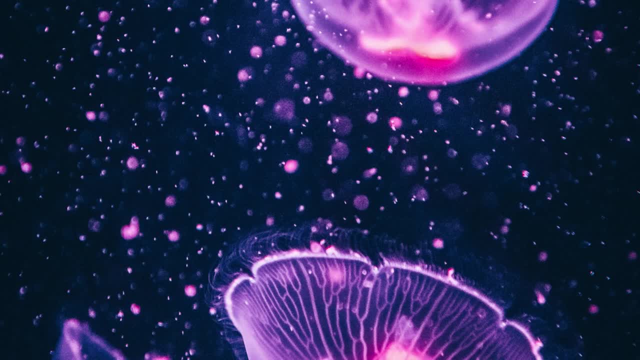 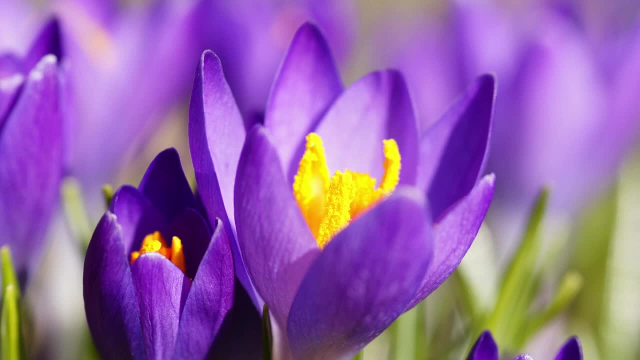 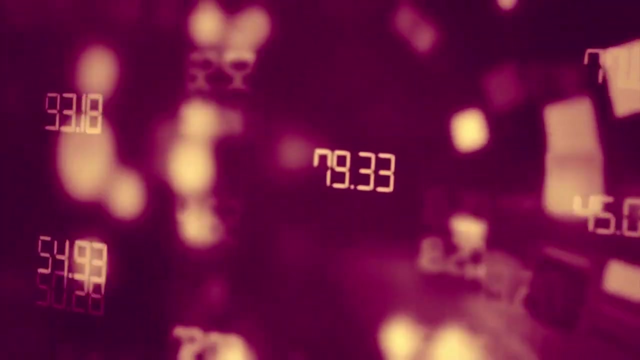 As you can see from this example below from Merriam-Webster's Collegiate Dictionary, in ancient times purple was considered a symbol of royalty. Purple is also used as an adjective to describe something that is expensive or luxurious. For example, I want my car washed in a fancy car wash like those ones you see on television. commercials where people are sleeping in their car wash. I want my car washed in a fancy car wash, like those ones you see on television commercials where people are sleeping in their car wash, Since people can't afford free water in their cars. so use the affirmative10, do you care? 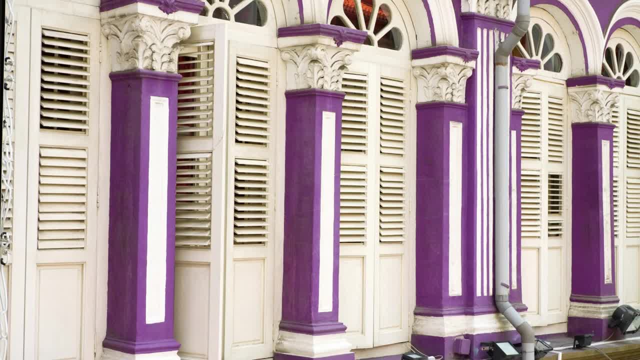 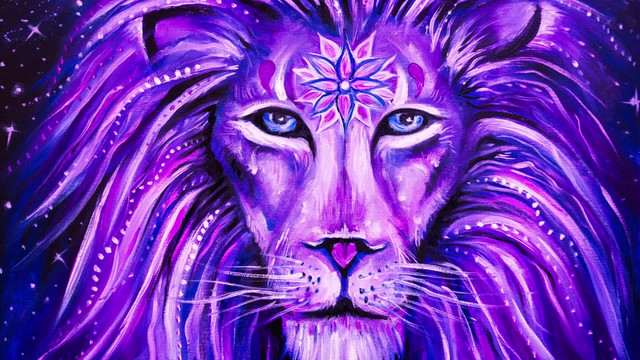 so just tell me, what was the reason they put a water bottle in there? Purple is associated with wisdom and spirituality. The color purple symbolizes the third eye, which is a spiritual center in our body that connects us to higher powers. It also represents knowledge and insight, as well as the ability to see things from 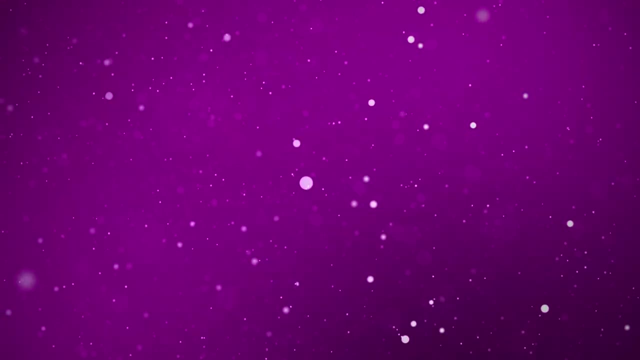 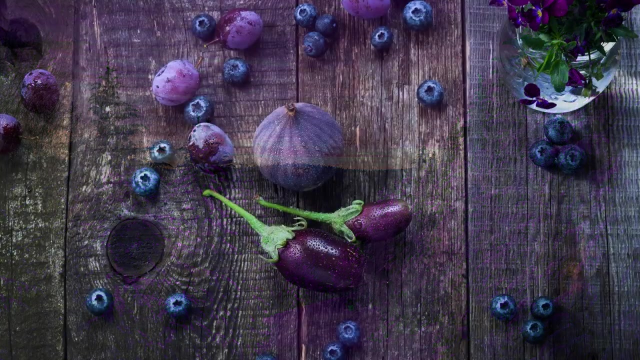 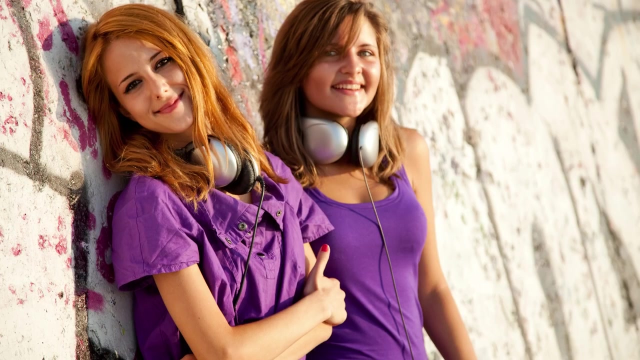 other perspectives. Purple's association with spirituality and wisdom makes it an ideal choice for your color scheme if you wish to explore the kilometers of life that are outside your doorstep from home, want your space to be more than just functional. You want someone who works there or visits to. 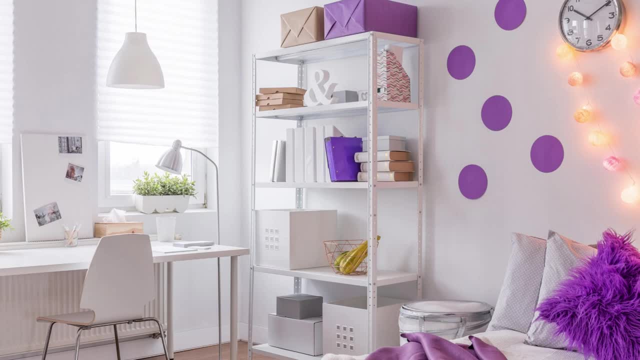 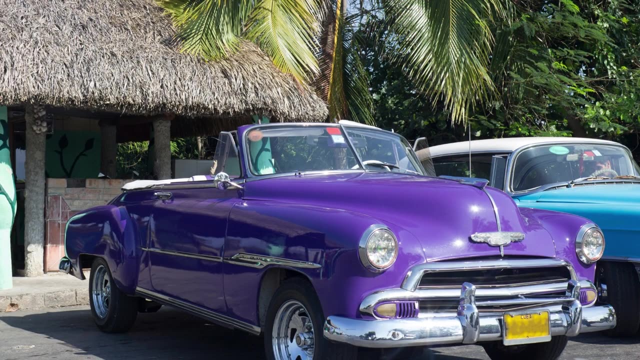 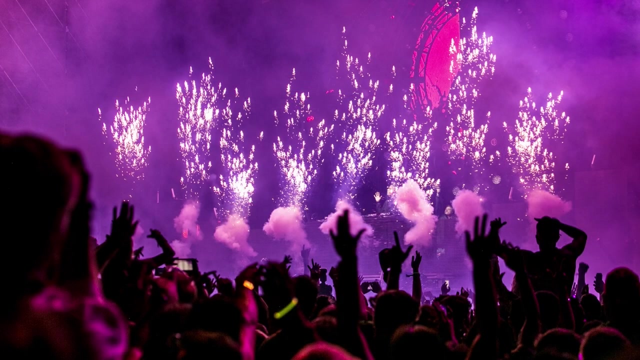 feel calm, relaxed and inspired by what they're seeing. Purple is associated with creativity. Purple is the color of creativity, imagination and dreamers. Purple is associated with magic in many cultures and religions. In ancient Egypt, purple was worn by royalty as a symbol of 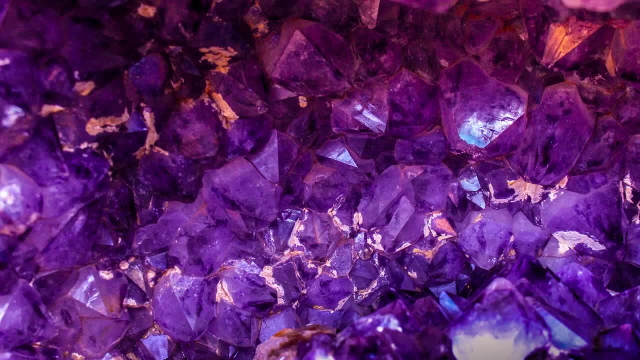 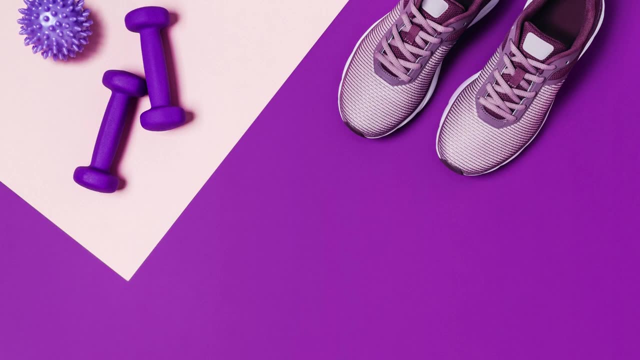 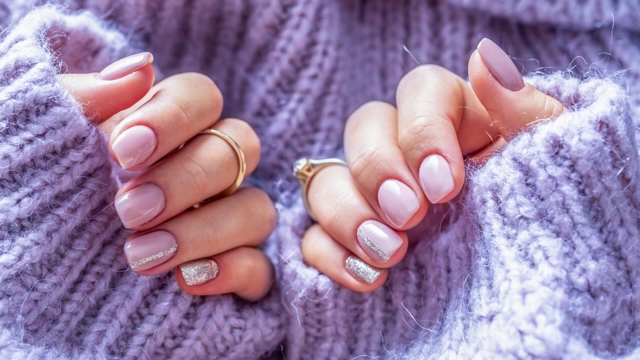 power and prestige. The Greeks believed that purple could be used to bring good luck or ward off evil spirits, or even heal illness or wounds. This latter belief may come from the fact that it was believed that certain plants grew exclusively in tropical regions. Purple has long been considered. 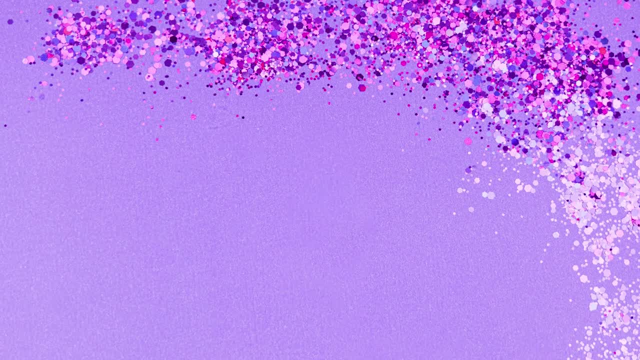 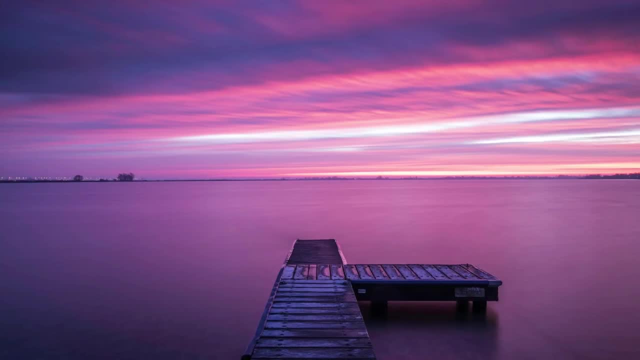 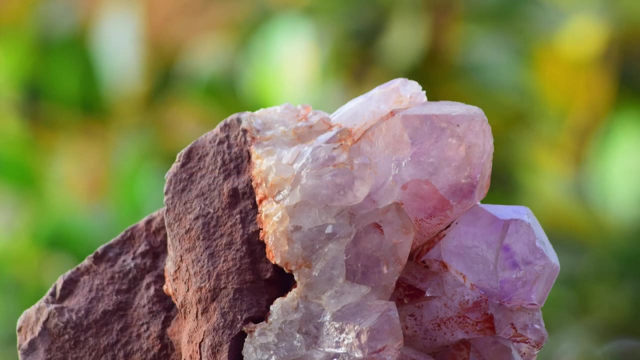 a mystical color, a symbol for magic, because it represents imagination and dreams. for mystery, because its appearance can vary depending on how you view it. for spirituality, because it often appears at funerals where grieving friends wear black clothes for privacy, together with white flowers which represent mourning while they hold hands tightly together. 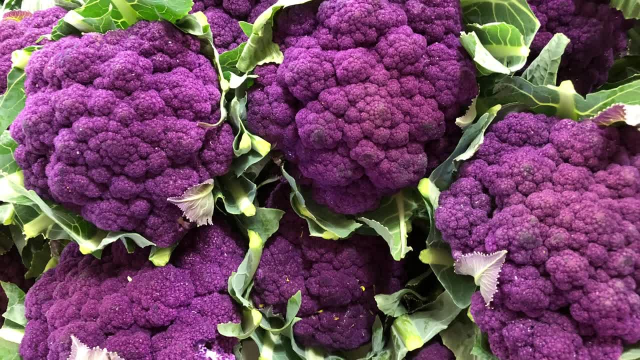 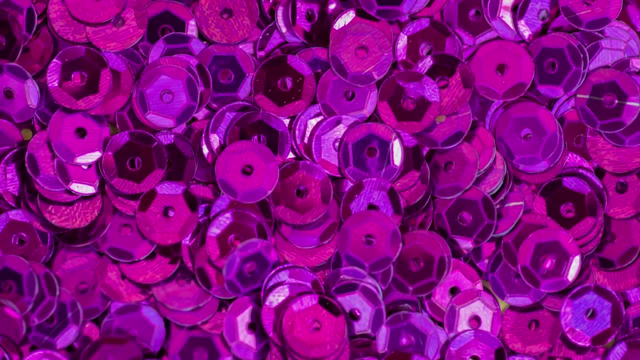 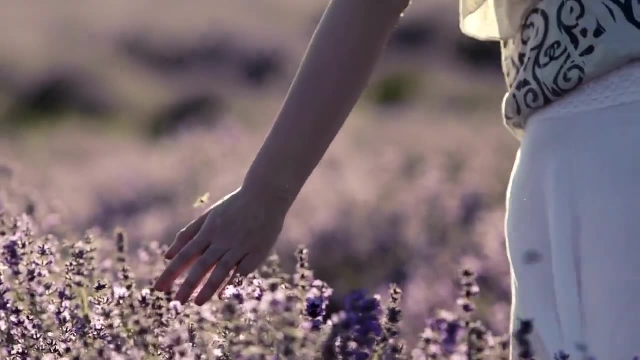 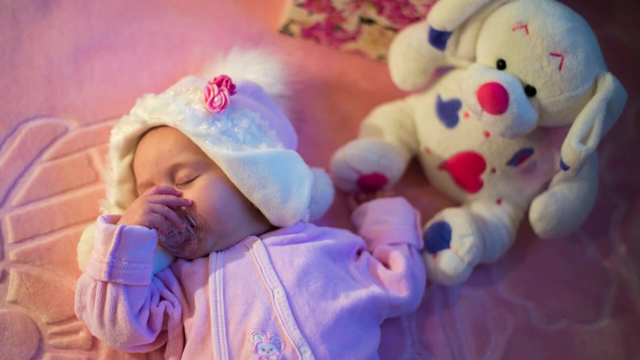 so no one else can see them cry openly. but what really makes this particular shade stand out is its unique ability to evoke feelings within people who see its vibrancy firsthand. Purple can be used to soothe the mind. Purple is a calming color. it can help you relax and sleep better. There are many ways to use purple in your home or office. 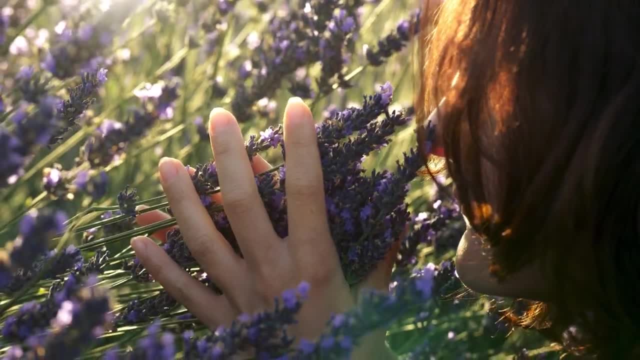 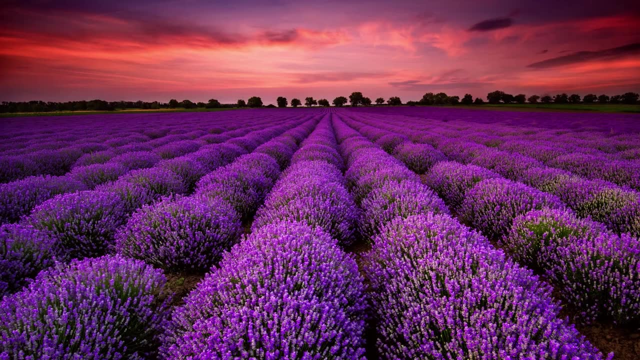 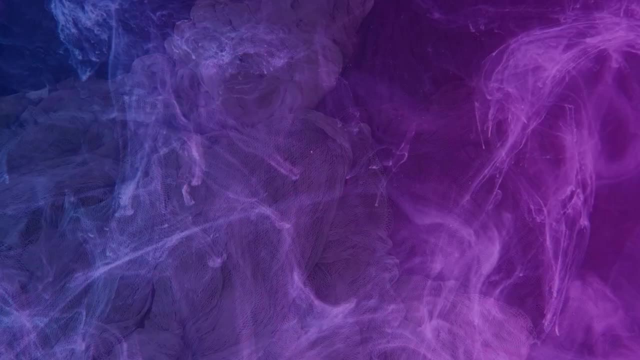 but one of the best is to have a purple rug next to your bed. Having this rug nearby will help calm you down when you're having trouble sleeping at night or simply want some privacy while reading in bed- Another way that purple has been shown to be effective at reducing stress and anxiety. 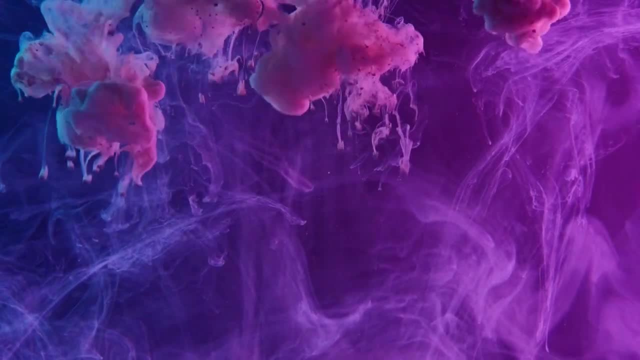 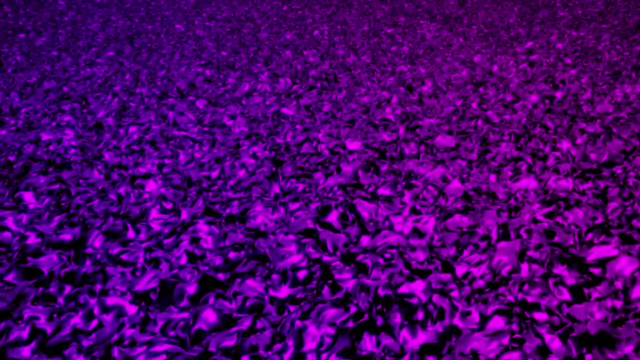 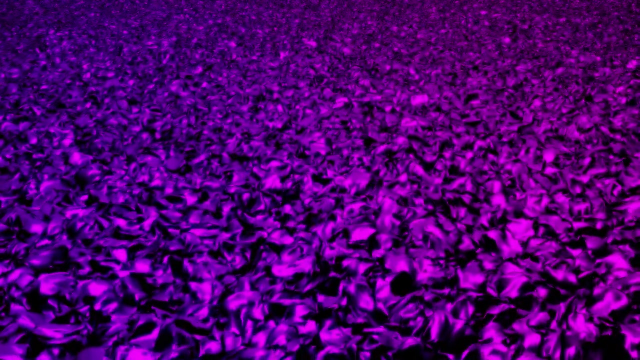 is through aromatherapy products, like candles made from lavender oil, which has been used for healing, which has been used since ancient times. Lavender also helps stimulate brain activity by boosting serotonin production, a chemical responsible for regulating moods throughout the body, and it's often paired with other 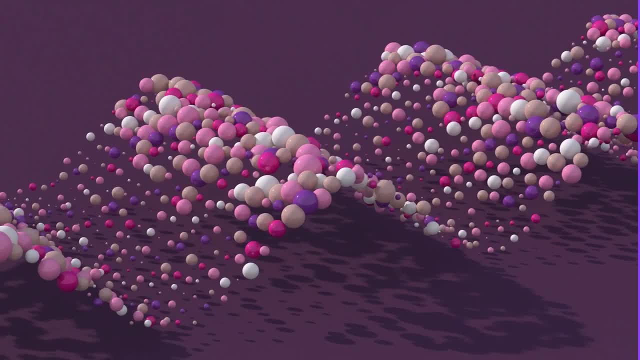 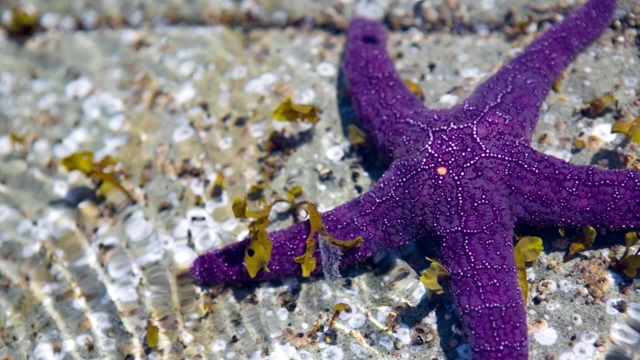 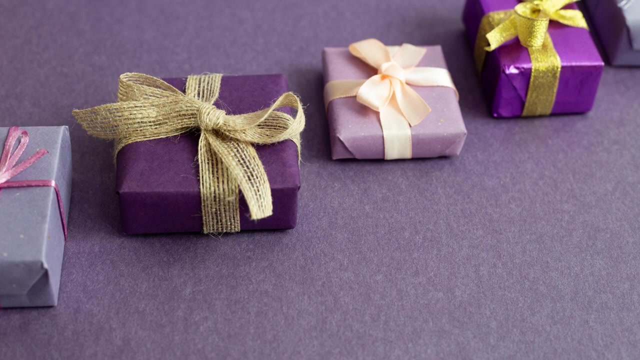 essential oils such as frankincense oil or violets, because they all share similar properties: Purple can be used to awaken the third eye. Purple is a great color to use when you want to stimulate your third eye. The third eye is the center of intuition and psychic ability. so if you're trying to 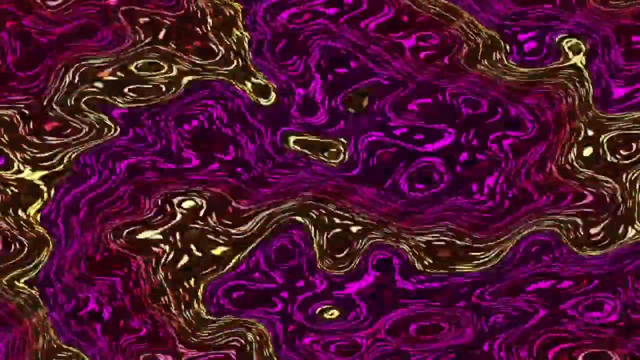 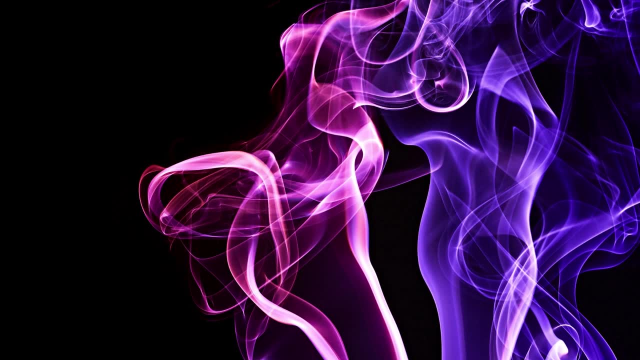 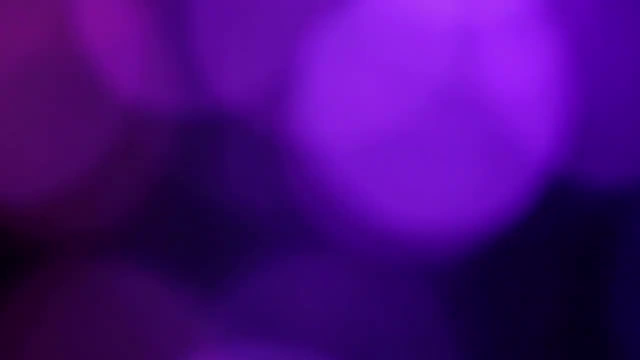 awaken this part of yourself with purple, it will be helpful. Purple has been used as a symbol for spirituality since ancient times and has many positive associations. It's associated with royalty and nobility. It's associated with virgin birth. It's an indicator that something is important or significant, such as a sign from God, ie.